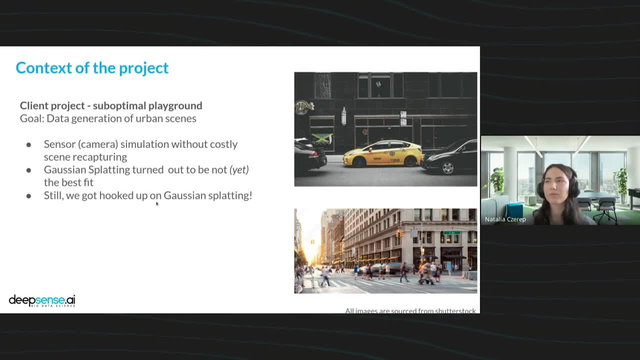 world model, some type of sensor simulation with the use of Gaussian Splatting and nerves. we were all in it. There are successful works from NVIDIA and WIMOD that build a world model on nerves for the urban scenes. We were inspired by their research and 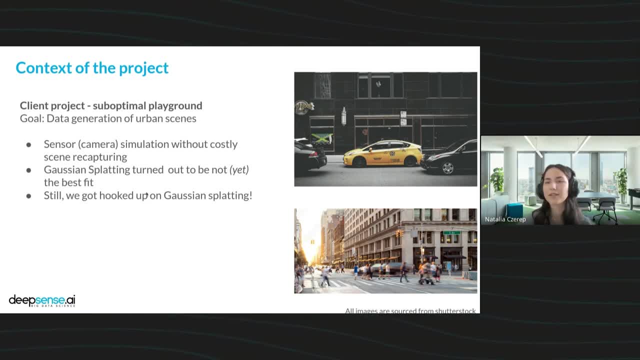 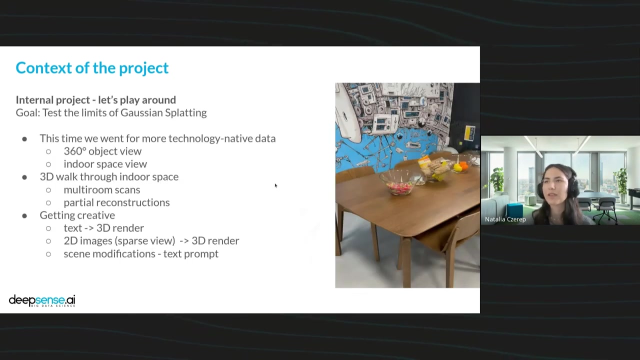 thought about the use of Gaussian Splatting. We thought it would be an even better choice, But it turned out that it is not an optimal playground for this technology. So we got hooked up on Gaussian Splatting and we proceed with our internal project. What we observed in the client's project was that 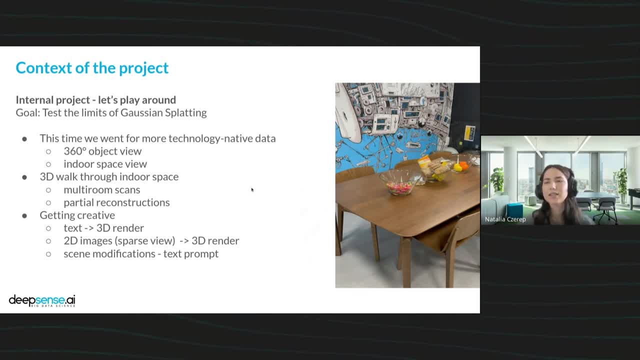 the urban scenes. the data is not really suited to showcase the method full potential. The urban scenes are very long. They have moving objects like cars or pedestrians. They are horizontal And most of the papers talking about gaussians or nerves consider 360 object view. 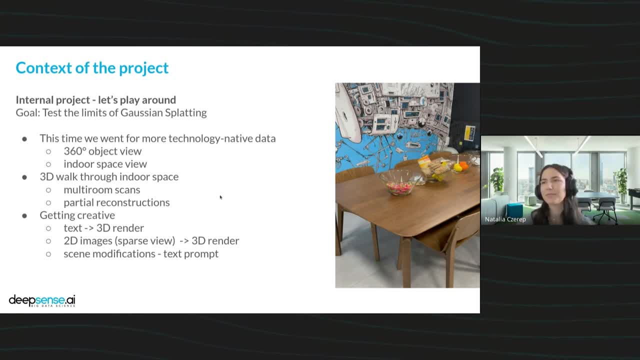 And it turned out that there is a reason behind it. So this time in internal project, we went for more technology, native data, let's say So. we tried 360 object view and we tried 3D walk through an indoor space. Besides renders, we got creative and we did some scene modifications and renders from text or from. 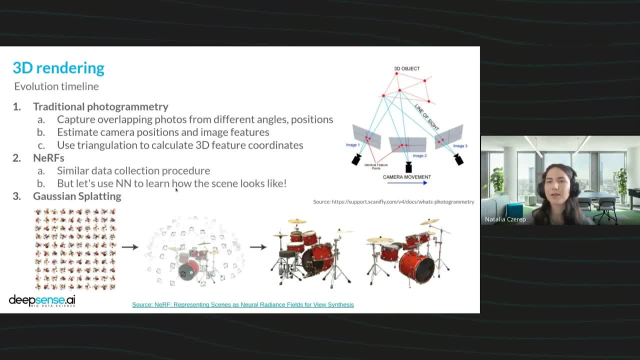 2D images. But before that I want to give you a short history note about the evolution in 3D rendering for some context. So we started with traditional photogrammetry, when it uses triangulation to calculate where the images feature. go, where to put the images features. 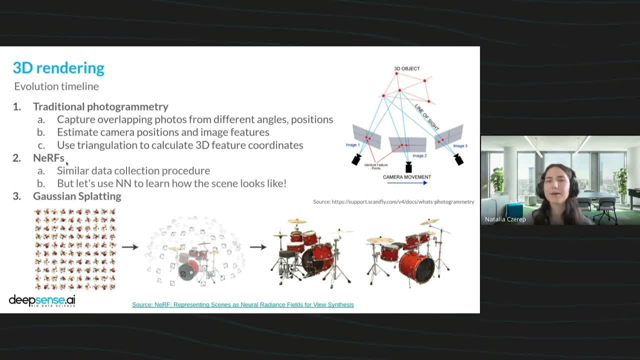 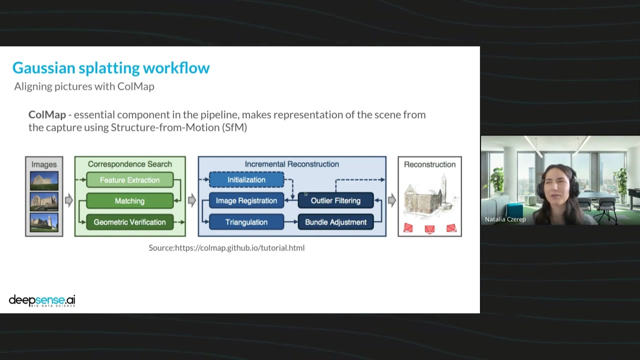 into 3D space. Then we got the nerves so we try to learn, try to make the neural network learn how the scene looks like. And then people got interested in Gaussian Splatting. But before we can train Gaussian Splatting we need a couple of information from the images. 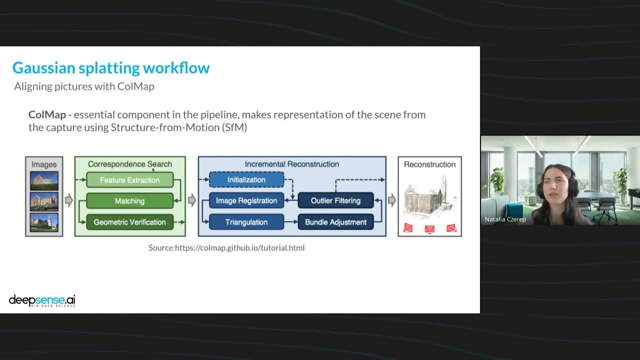 So in our experiment we used colmap and it provides the initial reconstruction of the scene from the object And basically what it does. its main task is to perform feature matching. So it extracted- extract just features from the map- Ok, different images- and match them and then use this triangulation to reconstruct. 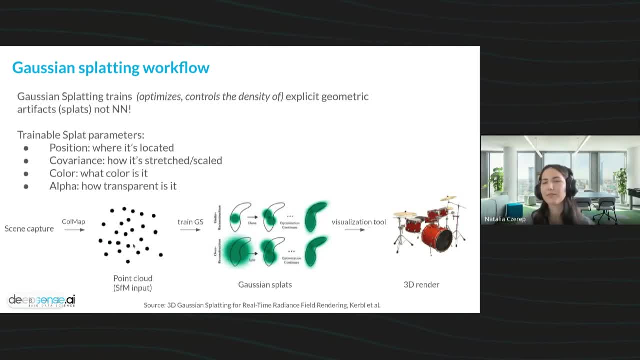 When we have the point cloud, when we have output from the call map, we can now train Gaussian Splatting. But when I say train Gaussian Splatting, I mean optimize its parameters, Because in Gaussian Splatting we have no neural network. we 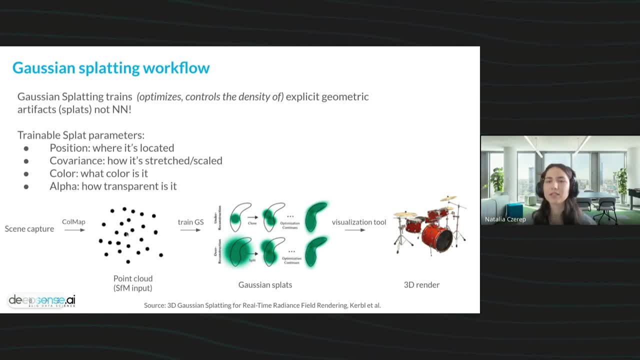 have explicit geometric artifacts, some ellipsoids, that we can optimize to cover our space To look like the object that we want it to be. So we can change parameters as position, so where the splat is located, how it's stretched. 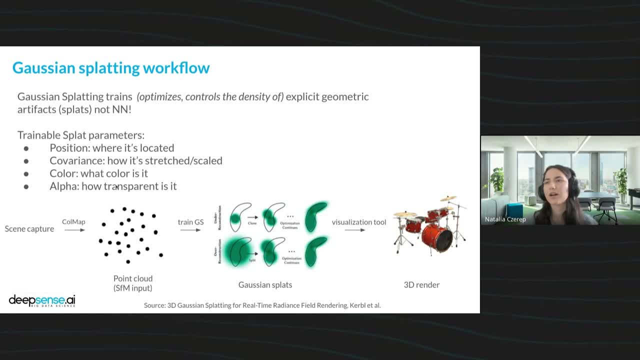 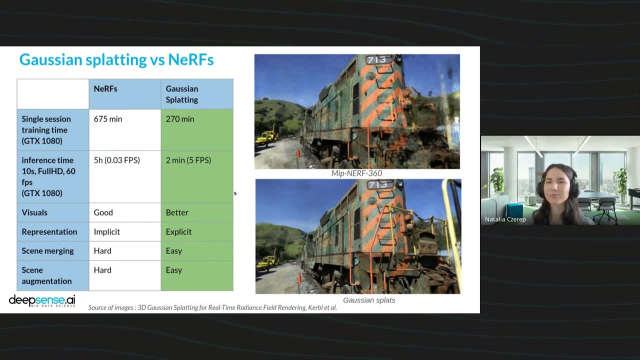 scaled, what color is it or how transparent it is. One can ask why we even started with Gaussians when there is already research on nerves, And I would like to say that we have a lot of experience with Gaussian Splatting And I would like to say that we have a lot of experience with Gaussian Splatting, And I would like to say that we have a lot of experience with Gaussian Splatting And I 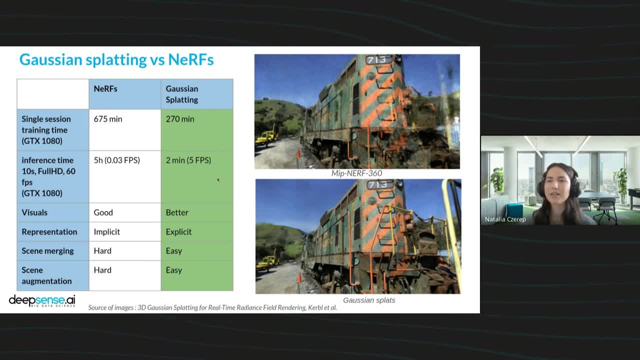 will let the numbers speak for themselves. So Gaussians are undoubtedly faster. They are written in this way. So that was that. But the visuals are better with Gaussian Splatting. What is more, they are not neural networks, so it makes them easy to be modified and controlled Because of the representation. 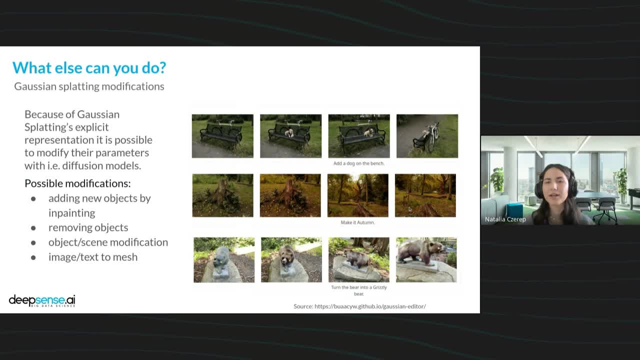 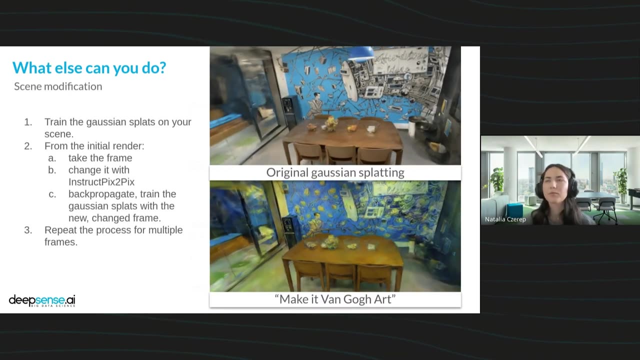 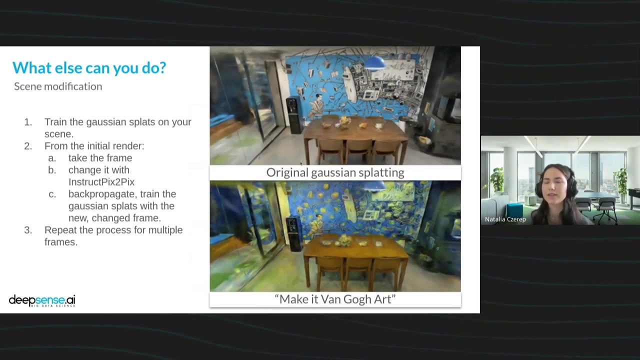 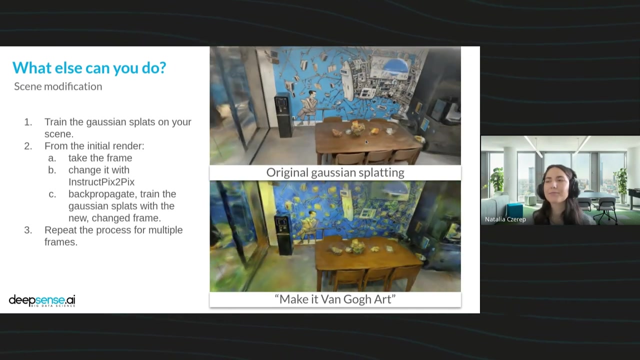 Gaussians are really easy to be modified, In example with diffusion models, So you can render a scene, render an object and change its characteristics by just a text prompt. What we did was scene modifications. So we had trained the initial Gaussians of our office kitchen And then we 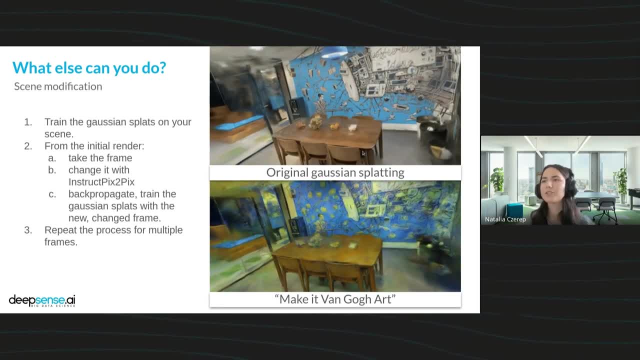 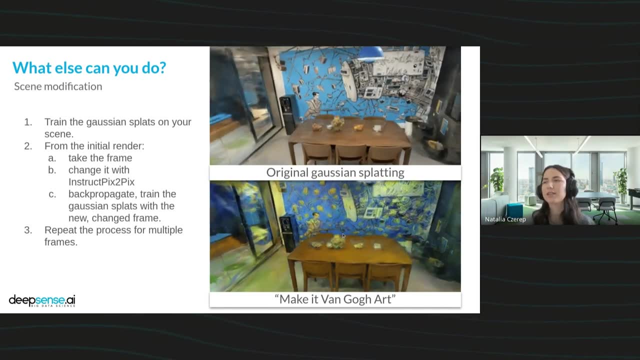 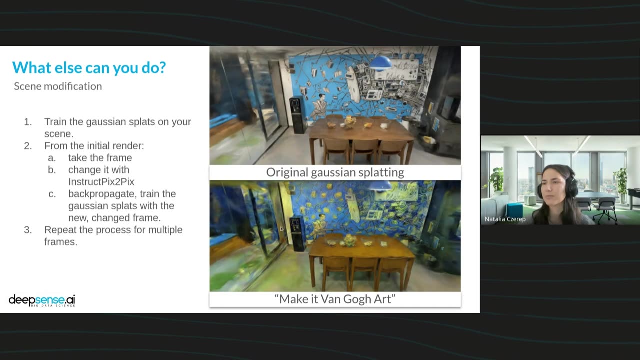 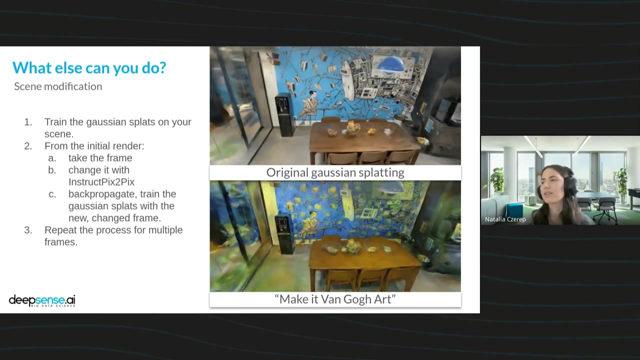 took the frame out of this render, changed it with InstructPix2Pix and then trained the Gaussian once again, trained the Gaussian Splats once again with the new change frames, And we did it a couple of times with multiple frames changed And, as you can see, the colors changed, The lines are: 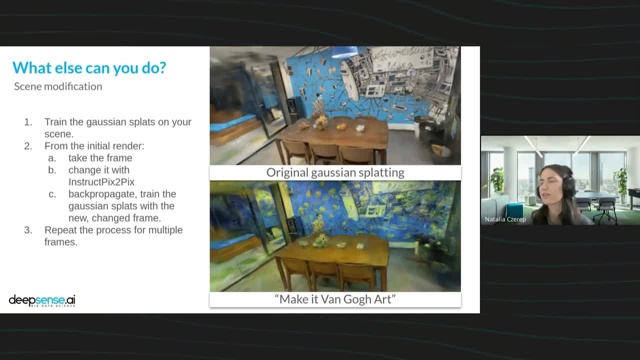 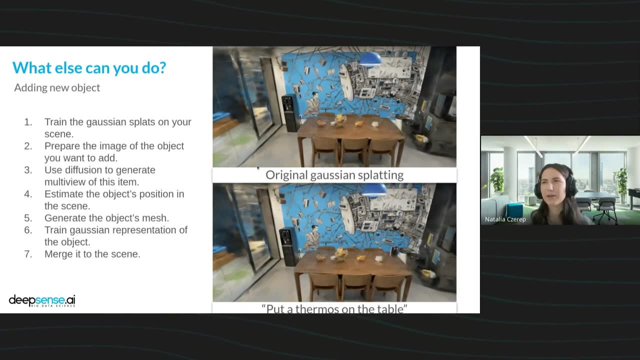 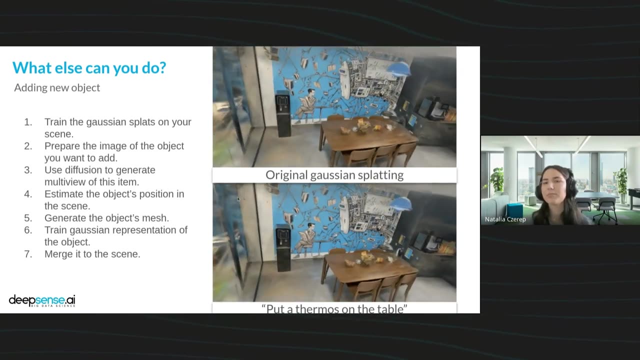 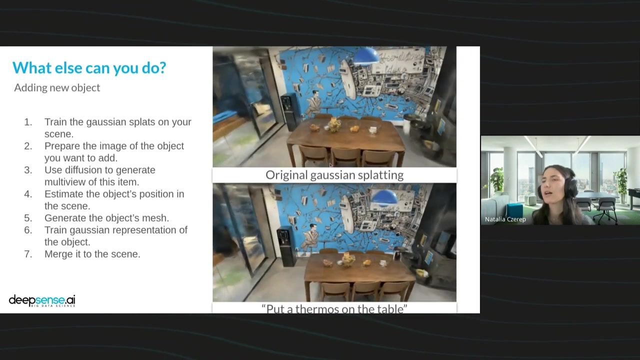 more like a painting, not so sharp, Yeah. So the next thing we tried to do was adding a new object to the scene. This time the pipeline was slightly different, So we trained the initial Gaussian Splats on our scene, Then we prepared the object. So we had one image. 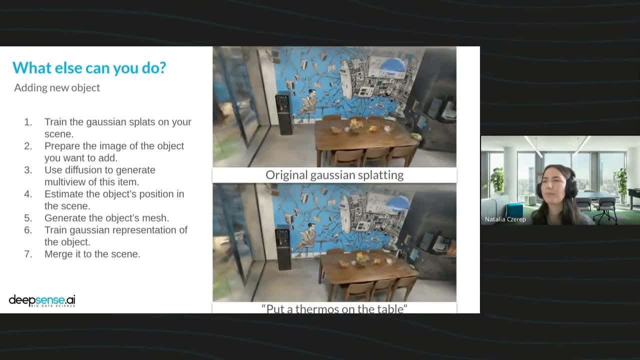 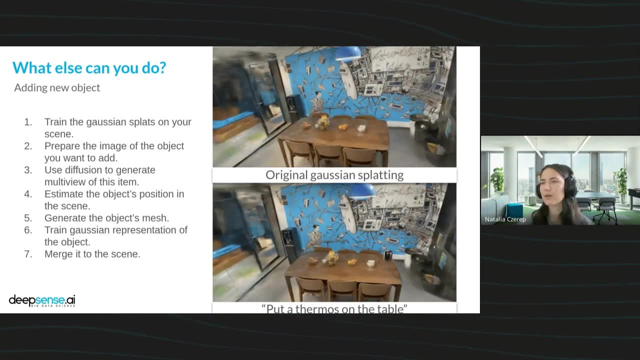 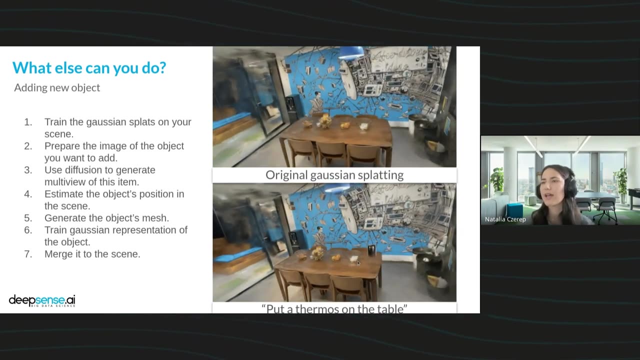 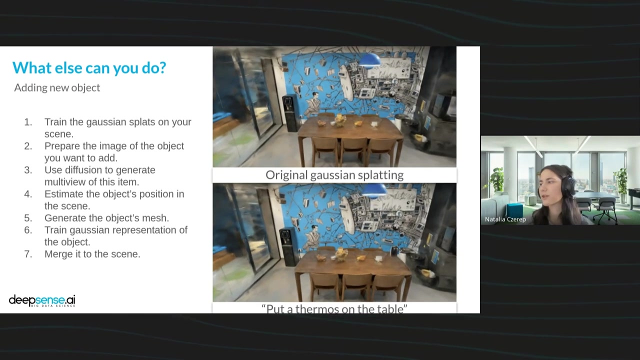 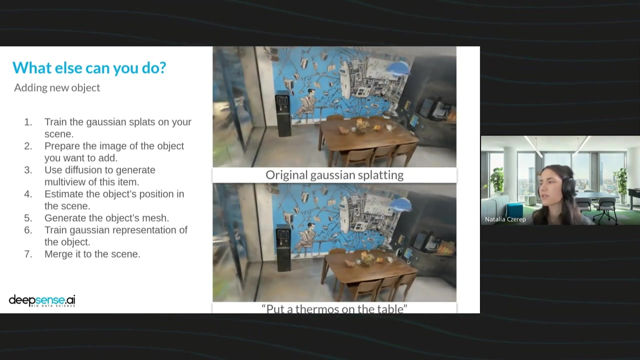 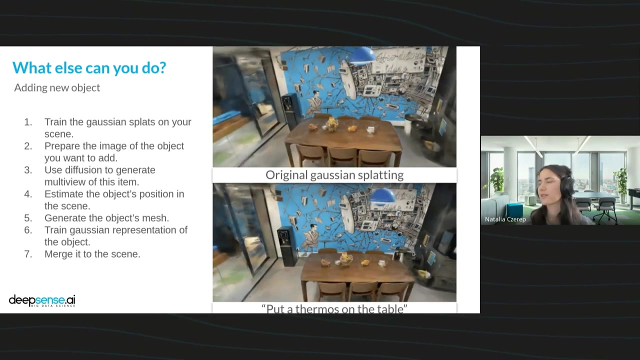 of our object And we, using diffusion models, generated different views of this object. We trained a Gaussian Splatting representation of the object And merge it to the scene So, as you can see, the thermos on the table can be seen in different angles. It's not disrupting background, So I think it looks. 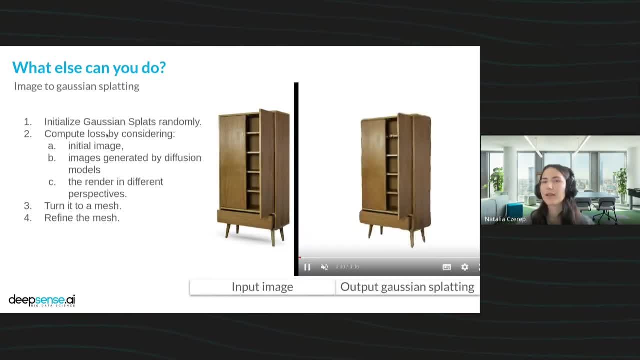 really cool. And besides changing the appearance of our kitchen, we also tried other techniques, such as Gaussian Splatting, generation from an image, from the text prompt or from mesh. There came in handy our experience with diffusion models, once again With the 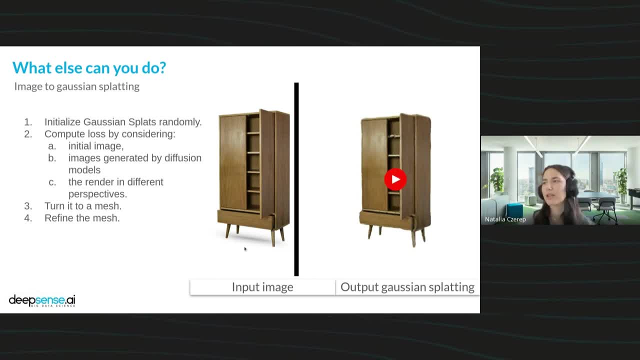 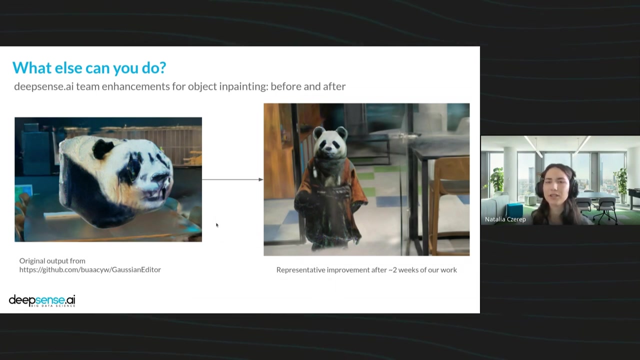 right initial capture, so just one image. we were able to do a Gaussian Splatting, So an render, 3D render- of this object, Everything thanks to a smart definition of the loss. As I mentioned before, the interest for the Gaussian spotting technology is growing now. 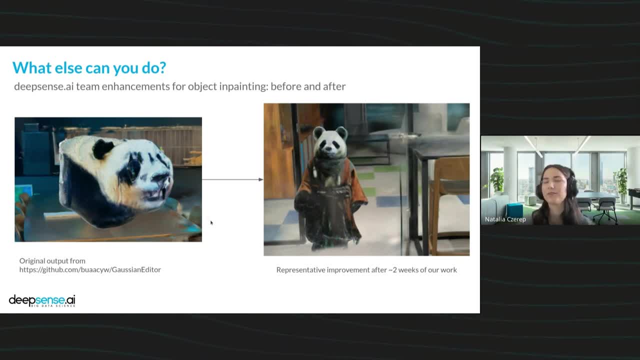 So the tools are not always perfect. The repositories grow in months So the results out of the box are not great. But with the little code tweaking our team was able to to work with that. So I think it looks very promising that it will only progress in the future. 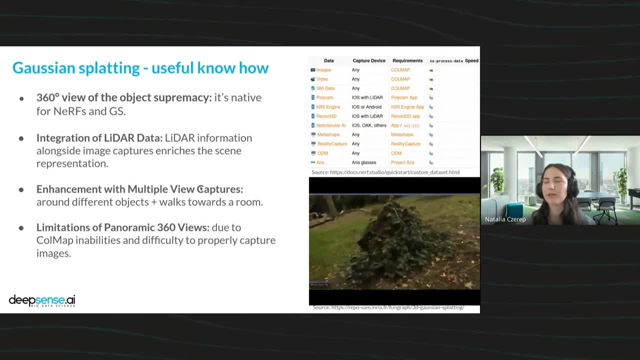 And when we come to an end, I want to share our thoughts and maybe useful tips for working with Gaussians. So first, when everyone is doing 3D, 3D rendering, we are able to get 60 views of an object And showing only that it's because of 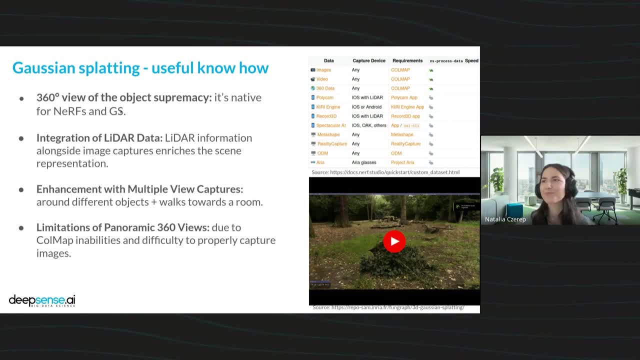 an reason It looks the best. Second tip would be: if you have LiDAR data, if you have depth information, use it. It can only benefit your render. When it comes to what we did with the, the indoor walks, we found out that going around the room is not enough.